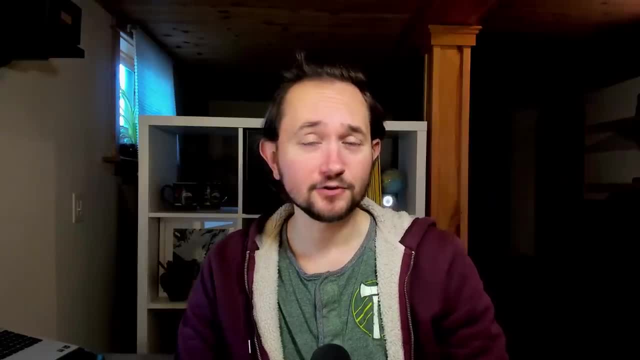 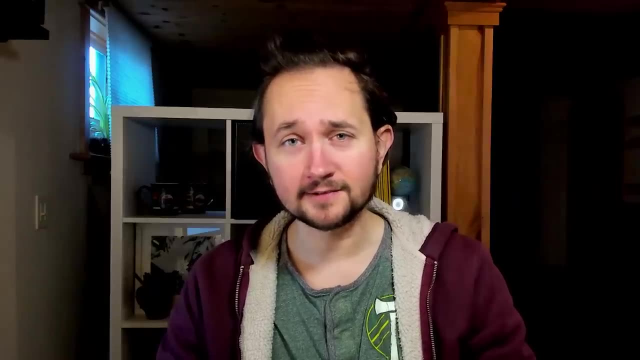 always been a North Dakota and a South Dakota, But there was nothing natural that split this territory in two. At one point, these two states were combined into a larger territory. Today, of course, that's no longer the case, And we're going to explore exactly how that. 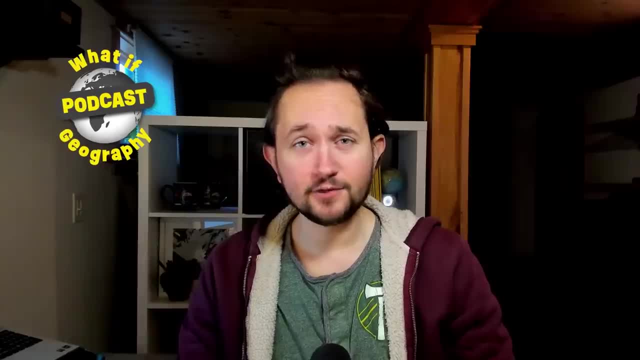 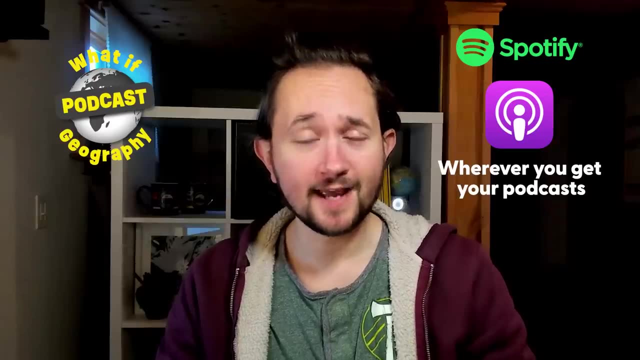 happened in today's episode. But before we get into why the United States has two Dakotas as usual, be sure to check out the What If? Geography podcast that I co-host with geography professor Hunter Shobie, If you enjoy geography and deep dives into complicated subjects. 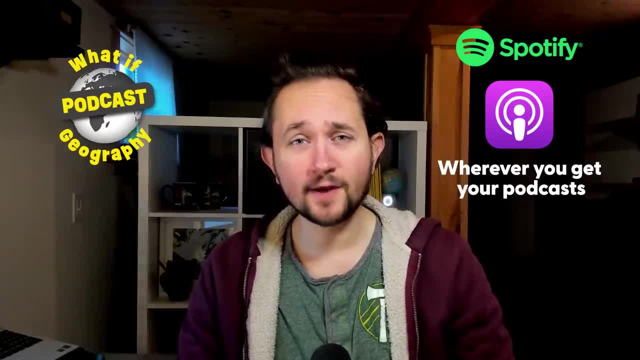 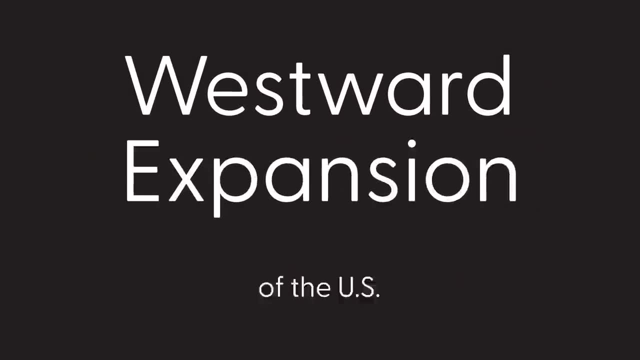 this is the one podcast for you. New podcast episodes premiere every Wednesday and you can get them right here on YouTube, Spotify, Apple Podcasts or wherever you get your podcasts. Before we get into the specifics of North and South Dakota, it's worth getting into a bit of. 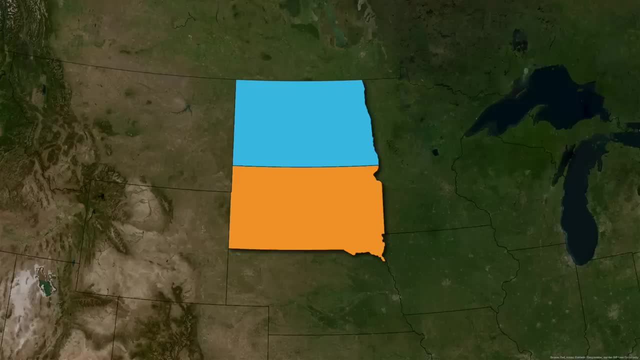 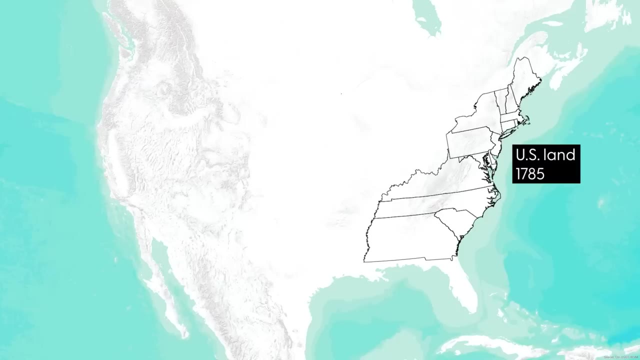 historic geography around how the United States expanded westward and how territories became states in the first place. Shortly after the conclusion of the United States War for Independence, the US was left with quite a bit of land that wasn't inhabited by citizens of the new country. 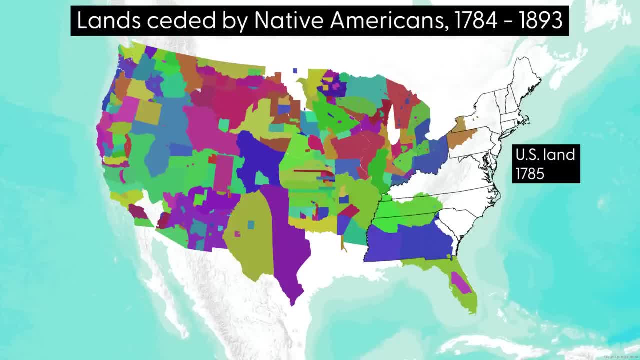 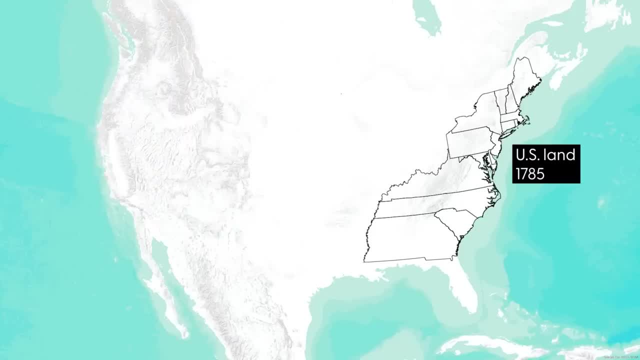 They were inhabited by a lot of Native American tribes, of course, and it's worth highlighting that these tribes would be systematically and brutally removed over the coming decades. But over the next 100 years the United States would grow from a relatively small area restrained to the East. 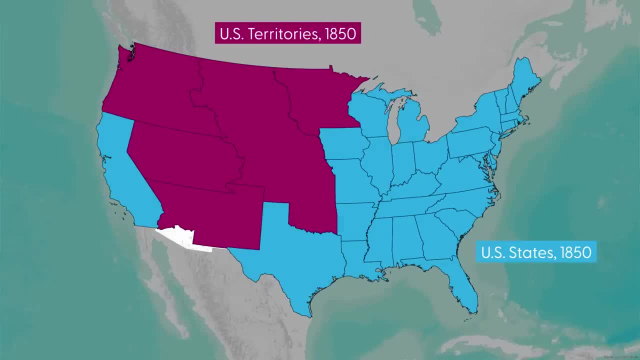 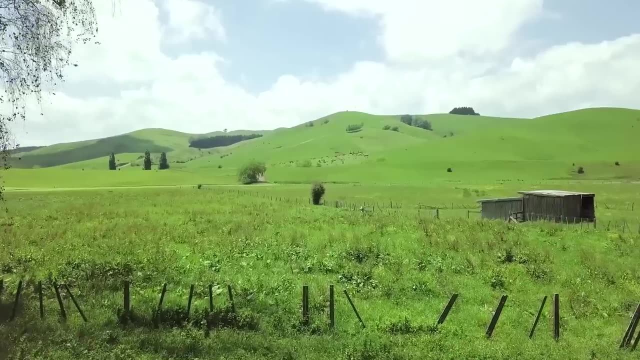 Coast to encompassing basically the entire United States we know today And as the United States grew, it had a fairly formulaic process by which it would organize the new land. The United States would send out a survey team to assess the land and, once complete, the land would be more formally. 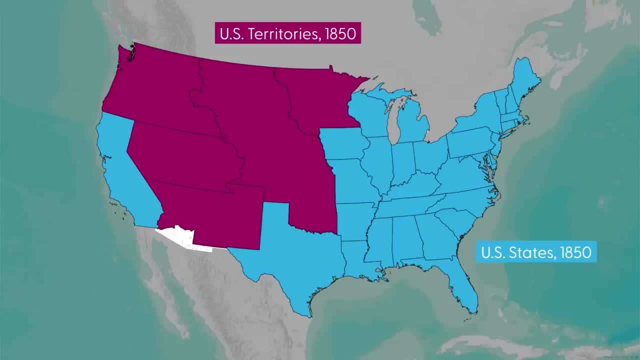 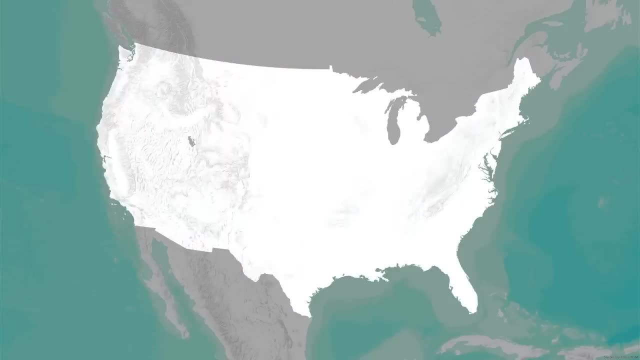 organized into a territory. These territories would have some form of territory that would be a territorial government, but otherwise would not have all the same rights and privileges of an official state. Now, territories could be all manner of sizes and proportions when they were formed. The Northwest Territory, for example, included the modern day states of Ohio, Indiana. 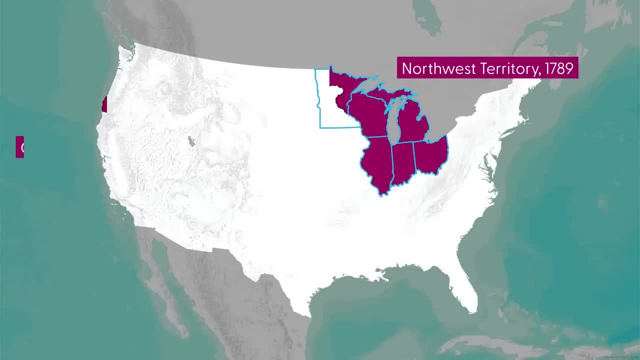 Illinois, Michigan, Wisconsin and parts of Minnesota. The Oregon Territory included the modern day states of Oregon, Washington, Idaho and parts of Montana, The point being that the way in which territories were originally organized was rarely the form they would continue with into statehood And the primary reason for why a territory would be split up. 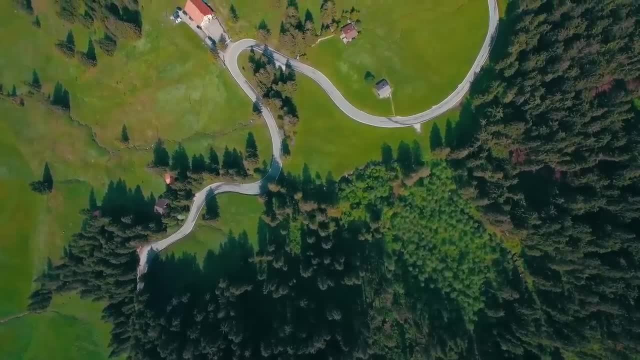 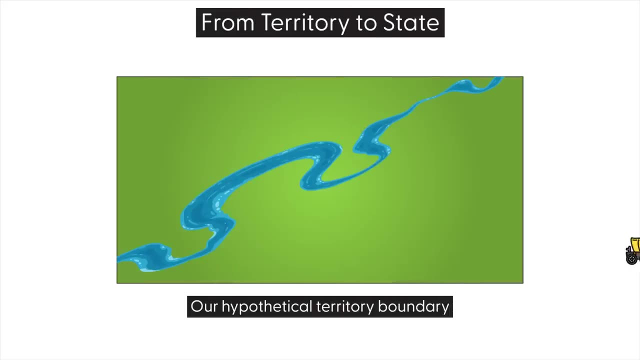 upon entering the country as a formal state was largely due to where and how the population that moved there was dispersed. As people moved into an area and cultivated the land, eventually, with enough people, they would request to be admitted into the country as a state. This was because they 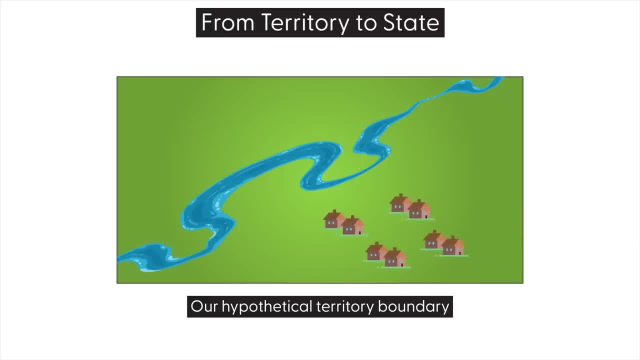 wanted those same privileges that other states got And, in order to do this, it required both houses of Congress to pass If one area of a territory was much less populated or geographically isolated. in order to make for a better argument for statehood, the people formally requesting: 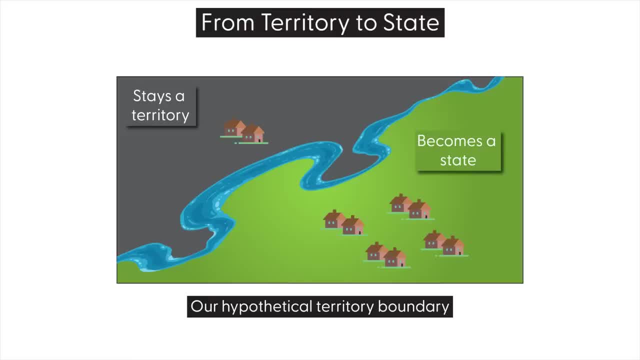 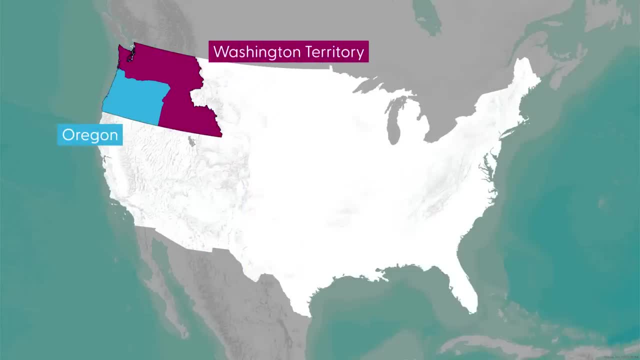 admittance would only request a smaller area become a statehood. So if a territory was a formal state, this largely occurred with many of the states we know today. Oregon and Washington, for example, were split at the request of the then-northern Oregon Territory. that felt like. 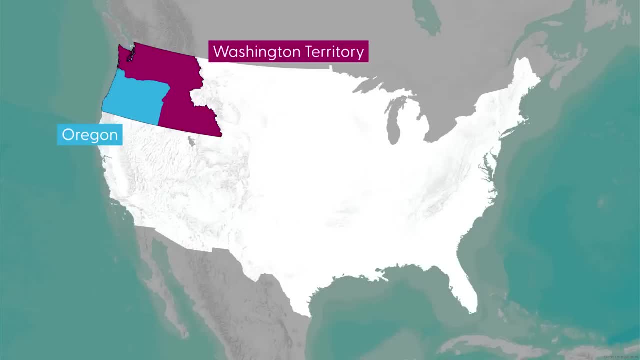 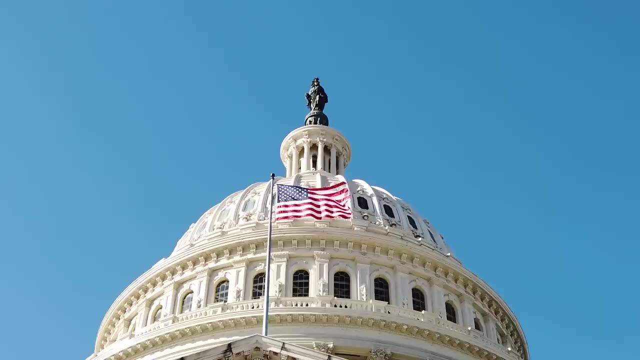 Oregon didn't represent their interests, At which point only Oregon was admitted into the union as a state. But while this was a common method for why a territory would be split up prior to entering, another method would boil down to one simple thing: politics. 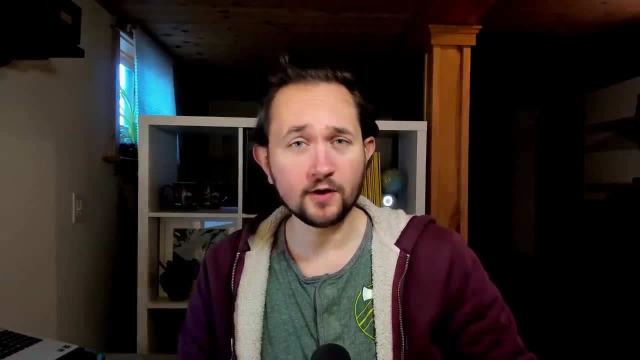 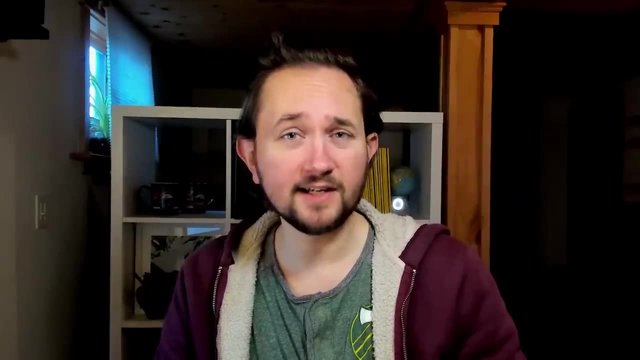 The current US state boundaries feel so permanent because we've all grown so accustomed to them within our maps and books. By the time that they were formed, most state boundaries were pretty arbitrary and, more often than not, politically motivated. But before we get into how North and South Dakota came to be specifically, if you're 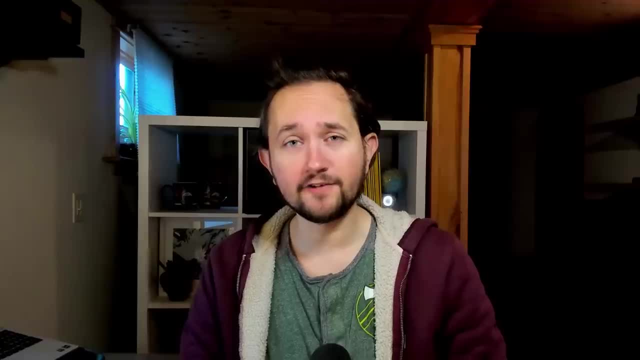 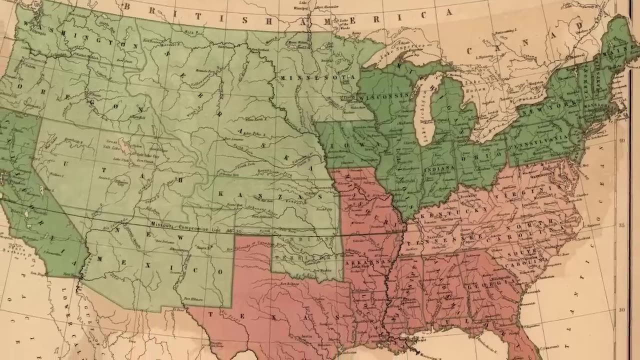 enjoying this video? hit that subscribe button. More fun geography videos are just a single click away. As we've already established, in the middle part of the 1800s there was an enormous push for settlement in the West by the US federal government. This, of course, came with the 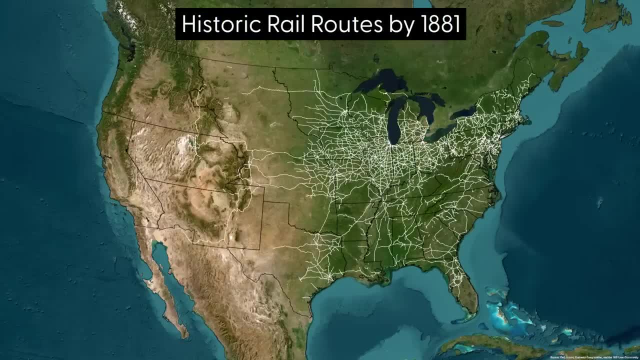 creation of new train routes to move people and goods quickly and efficiently to the country's newest territories. Unfortunately, during this time, train routes weren't often built going north and south within these new territories. The goal was always to connect people with population hubs back east. 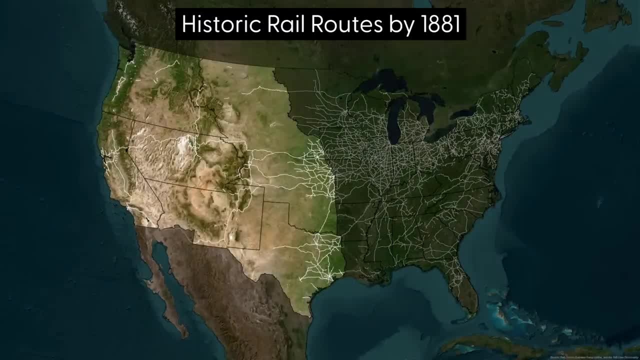 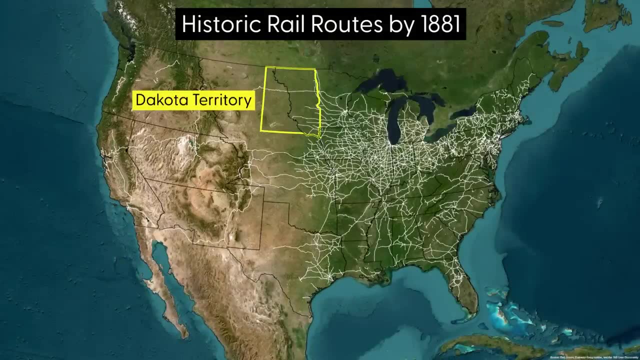 not with other population hubs in the frontier Which, to be fair, any population hubs in those days were rather small, so there was little reason to spend big on rail to connect them. In the case of the Dakota Territory, it had two primary rail routes moving through it. 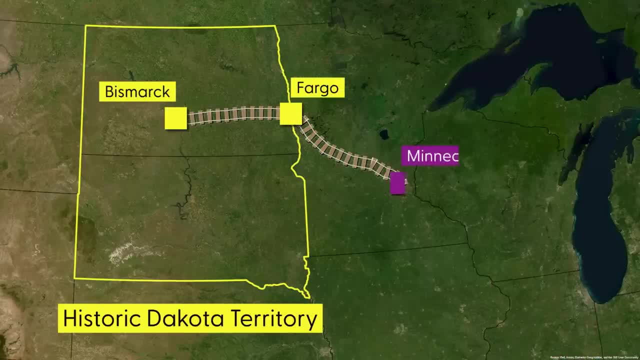 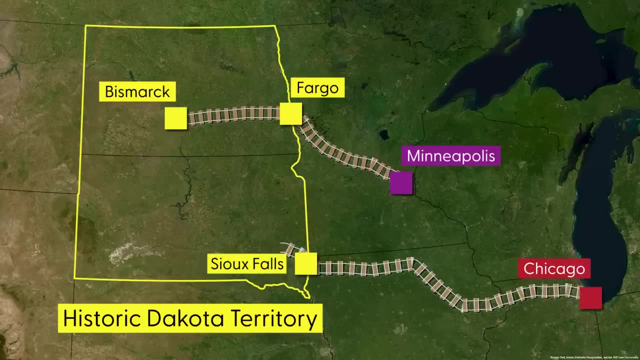 In the north, a train connected to Minneapolis by way of Fargo. In the south, a train connected to Chicago by way of Sioux City. That might not seem like a big deal, but it was a big deal. But remember, back in the 1800s Minneapolis was a relatively small, agrarian-focused city. 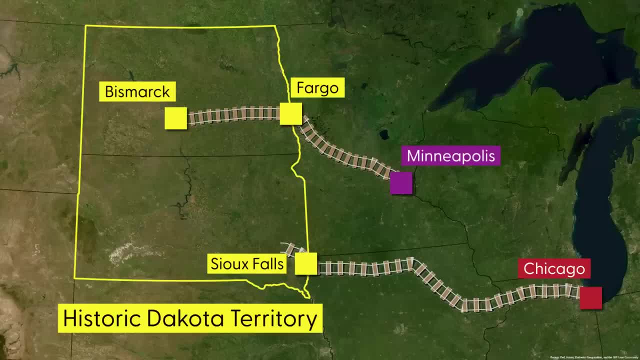 whereas Chicago was the big metropolitan city for the region. With far more movement between these two regions to the northern and southern parts of Dakota respectively, it's not that surprising that differences began to emerge between the two sets of people. And, as with any region, there are bound to be differences in how each are settled and managed. 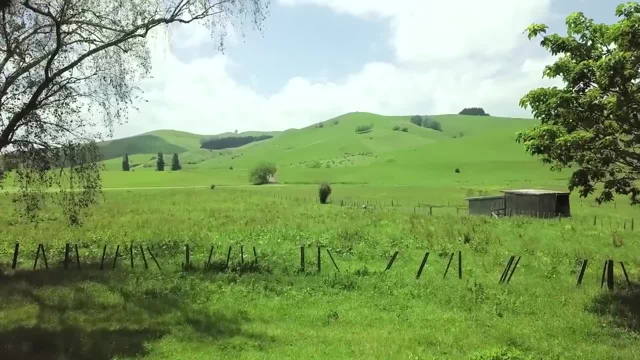 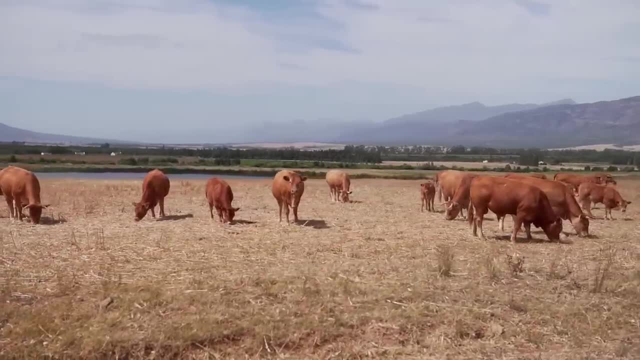 In this case, the northern portion of the new territory began developing in a more rural fashion than the southern half: Cattle ranching, fur trading and far more agriculture per meated. the northern portion of the territory whereas the southern part was more populated. 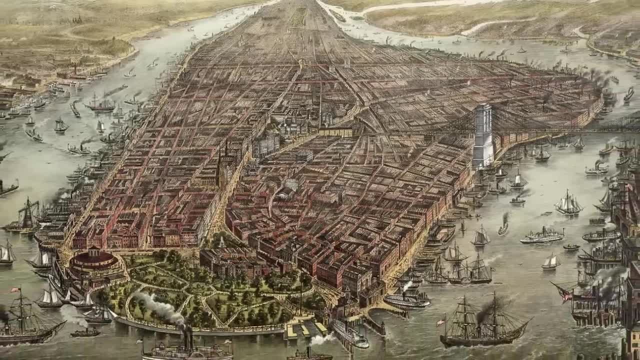 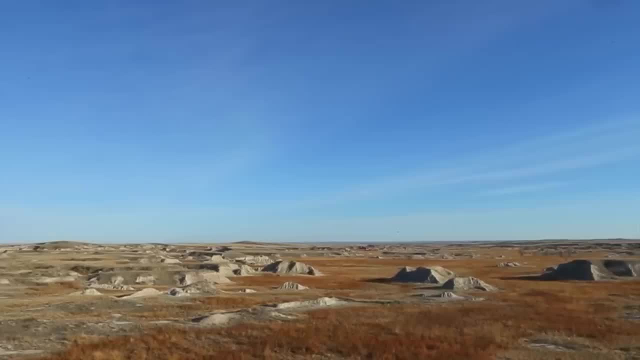 and far more urban-oriented. Nothing like New York City or Chicago, of course, but certainly more so than the north. This started the original cultural deviation between what would become the north and the south. But the differences between the two halves of Dakota weren't just. 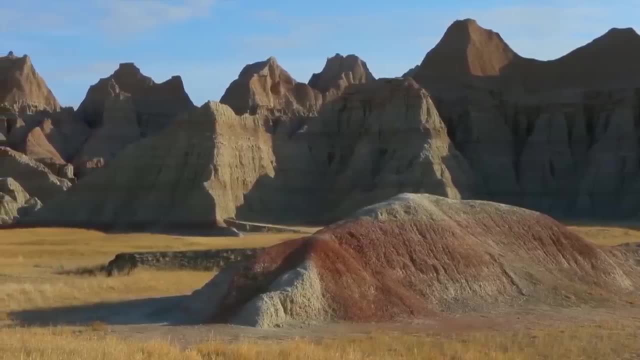 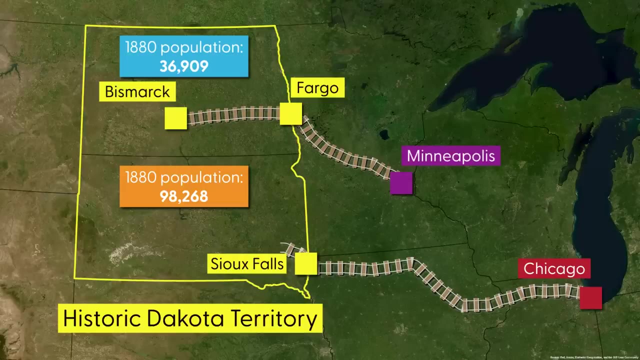 based on cultural opinions. There were tangible aspects at play as well. The southern part of Dakota had a population roughly three times the size of its northern half, and those in the south desired to become a full-fledged state, given that they met the population requirements. 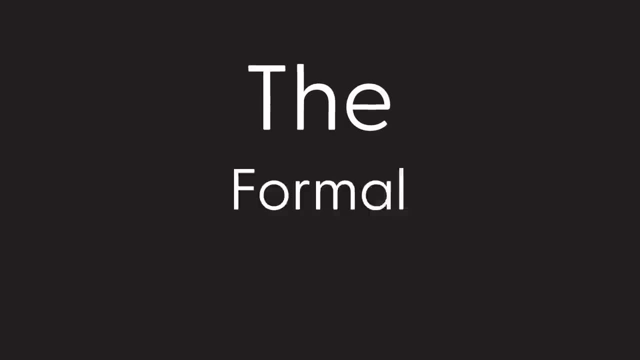 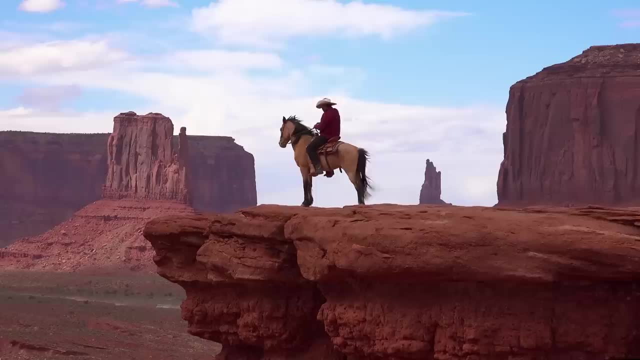 beset on them by the federal government, So in this case, the northern portion of the state was the federal government at the time. While everything we've covered is important cultural context and builds to an inevitable split, the real reason why we have two Dakotas today is something far more superficial During 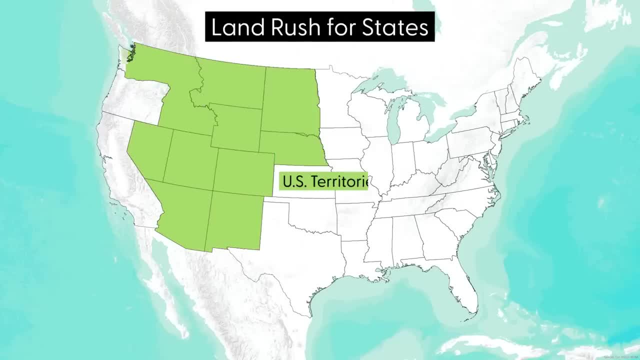 the mid-1800s, there was a bit of a land rush in terms of getting territories converted into full states, And if you were the party that was in control at the time, you had considerable power to shape whether you were going to allow a new state that would vote your way or not. 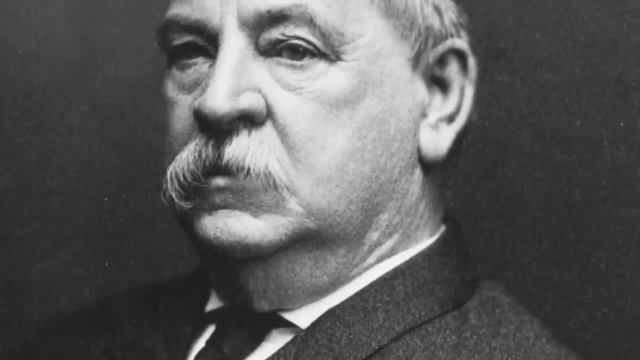 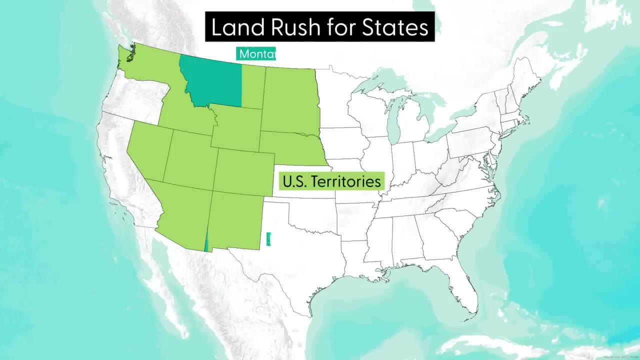 In the case of the Dakotas, the president at the time was Grover Cleveland, a Democrat, and in 1888, President Cleveland proposed admitting four new territories as states: Montana, New Mexico, Dakota and Washington. His logic was the former two states would. 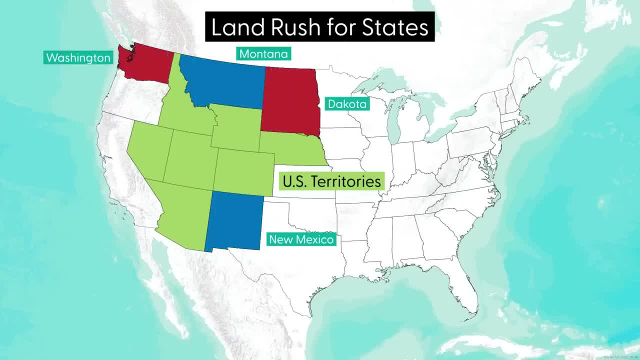 vote Democrat and the latter two would vote Republican, and therefore it should be an easy pass within a split Congress. Unfortunately for Cleveland, later that same year, Republicans gained majorities in both the House of Representatives and Senate, which changed the equation quite. 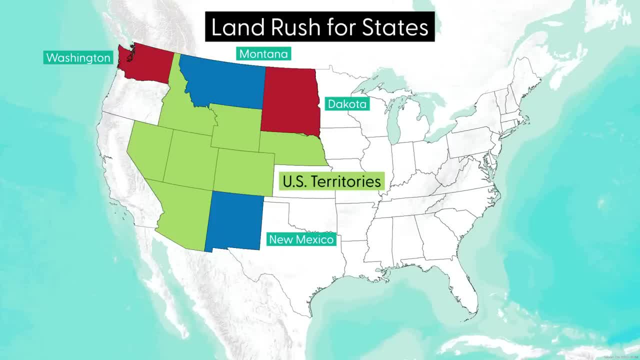 a bit. In order to get ahead of the possibility that a Republican-led Congress would only admit Republican territories into the union, Congressional Democrats were allowed to vote in the House of Representatives and in the Senate In order to get ahead of the possibility that a Republican-led Congress would only admit Republican territories into the Union. Congressional 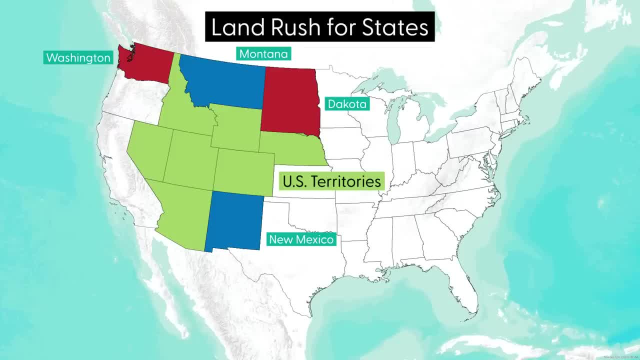 Democrats cut a deal with the Republicans to allow for Montana and Washington into the Union, but not New Mexico. And, of course, given that there had already been multiple attempts to split the Dakota territory prior to this moment, Protestants seized on the opportunity to split not just Dakota but two territories and admit both at the exact. 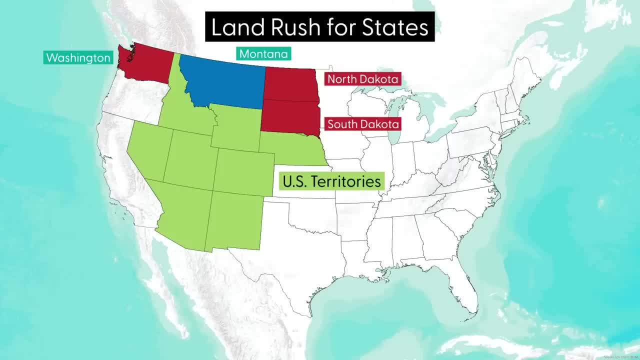 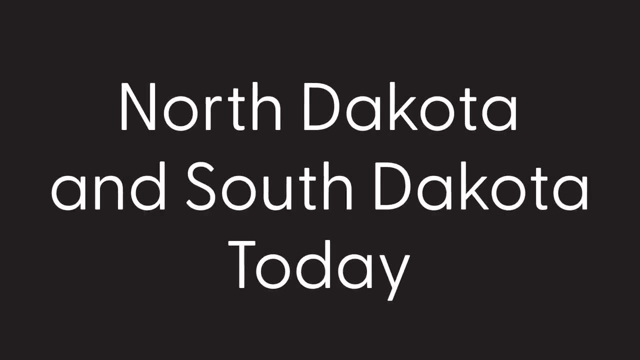 same time. All in all, the Republicans managed for three Republican states and for this at just a single Democrat state, Outro. Today, of course, we have two Dakota states states- North Dakota and South Dakota- and they are very similar to each other. There are some. 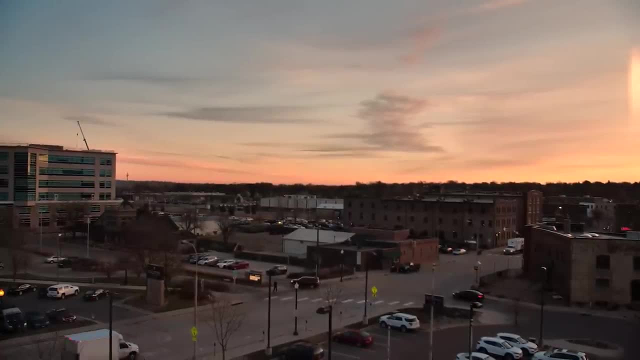 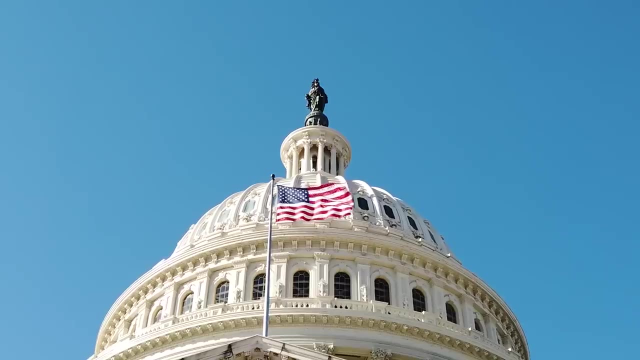 minor differences here and there, but largely within the context of the United States, they're basically the same. This is perhaps not all that surprising, given that the two states are literally right next to each other, but it can't be understated that the Dakota territory was split. 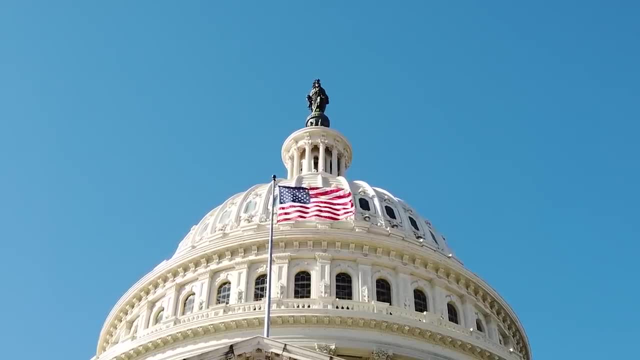 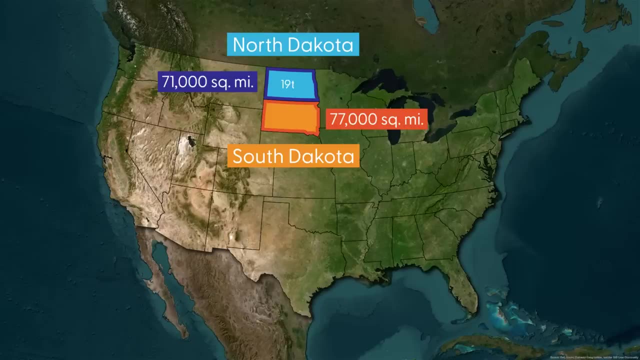 up for political reasons, not natural or even cultural ones. Both states are very similar in size. North Dakota is about 71,000 square miles and South Dakota is about 77,000 square miles, making them the 19th and 17th largest states respectively, If we pulled the two states. 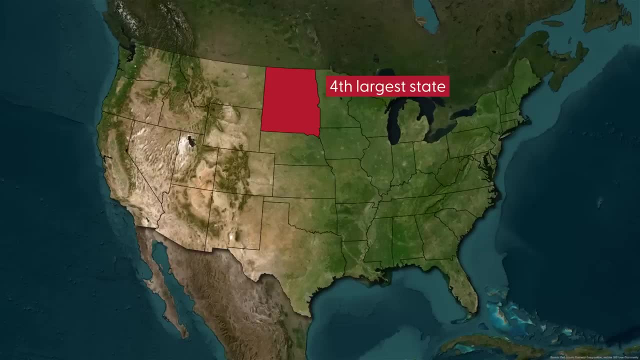 together they would become the fourth largest state, by just a few hundred square miles behind Alaska, Texas and California, and almost exactly equal with their neighbor, Montana. Additionally, both are fairly rural even to this day. North Dakota's largest city is Fargo. 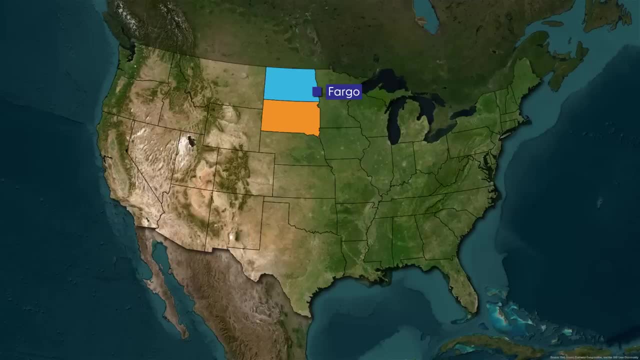 which has about 252,000 people within the entire metro area, and South Dakota's largest city is Sioux Falls, which has about 282,000 people In total. each state only has three US Census Bureau-defined urban areas With a handful of urban clusters. this leads to North Dakota as being about 40% rural and 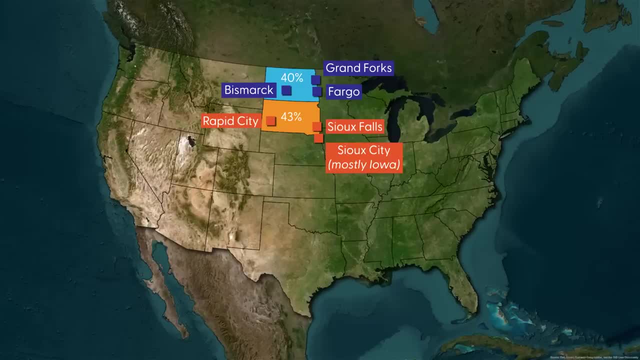 South Dakota at about 43% rural. To put this in perspective, the US rural population stands at about 20%, And not only are both states heavily rural, but they're both very conservative in their politics. As of today, both states have a Republican governor and lieutenant governor. 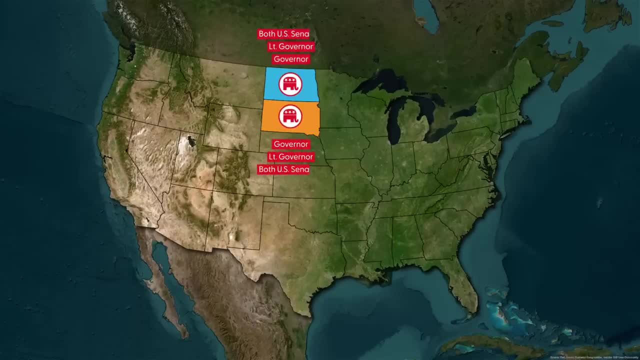 Each state's two US senators and single US representative are both Republican, And both states' legislators are heavily dominated by Republicans. On a political level, the two Dakotas look exactly the same. Finally, even the two states' climates are fairly similar, though North Dakota can get quite a bit. 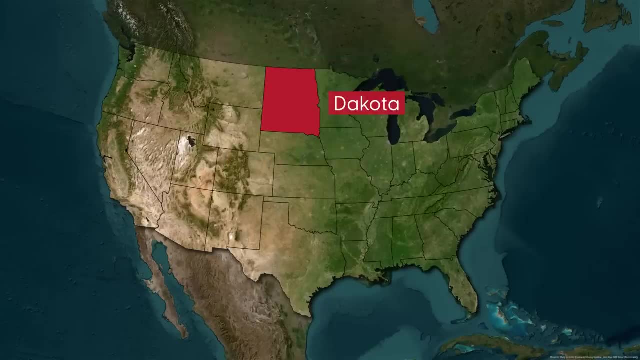 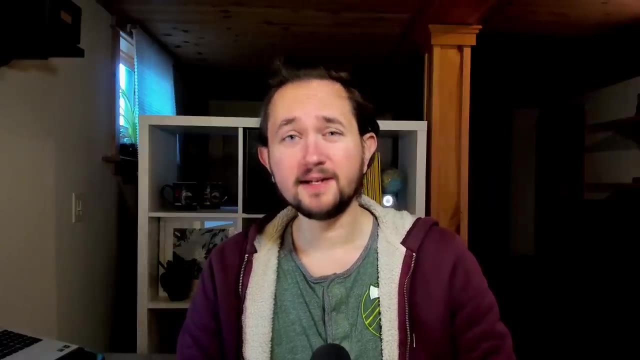 colder. All this is to say. had North Dakota and South Dakota started out as a single state, there likely wouldn't have been anyone suggesting it should be two states. today, The Dakota Territory probably should have been admitted as a single state. But as the saying, 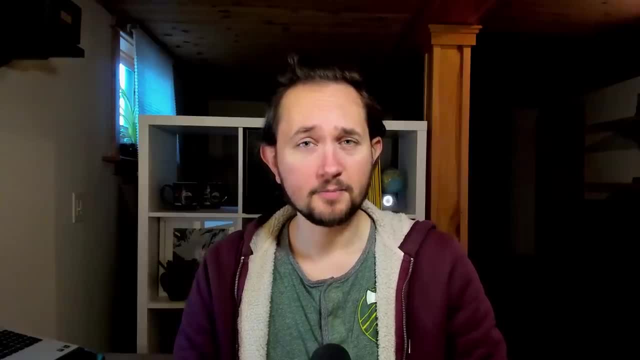 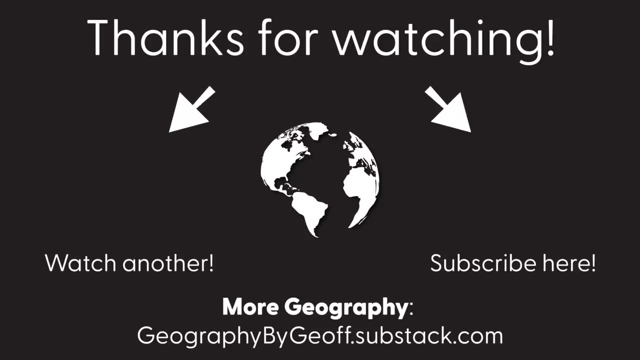 goes all's fair in love and war. In this case, the Republican Party was able to shrewdly get two states in the place of one, much to their great benefit in Congress today. I hope you enjoyed learning more about the Dakota Territory. 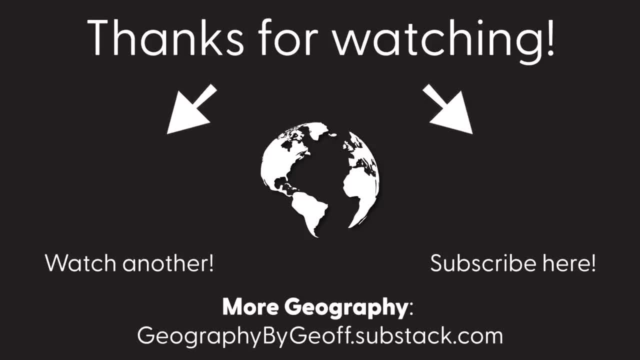 and how it came to be two separate states. If you did, please subscribe to my channel, And if you want to watch more of my videos, you can do so here. Thanks for watching. See you next time.